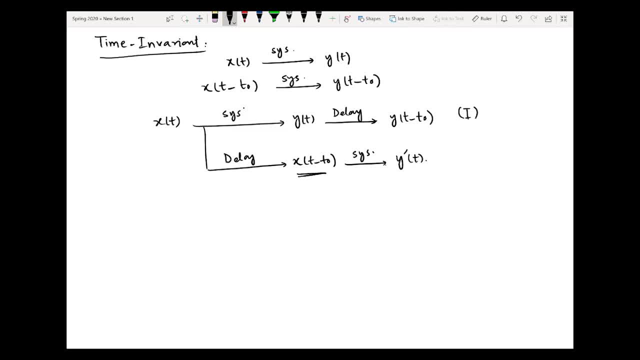 dash of t because the input is changed. so if I change the input, the output will be definitely changed. now we can have two cases. if this y dash of t is equal to y of t minus t naught, which is the first result, it means that the system is time invariant. and if this white 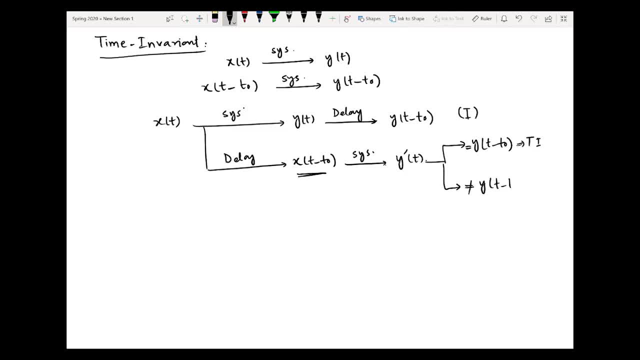 prime of t is not equal to y of t minus t naught, then this case, the system will be time variant. so we have to simply check this flow in order to verify the time invariance property. again, we can have two examples to have further understanding of this concept. so the first: 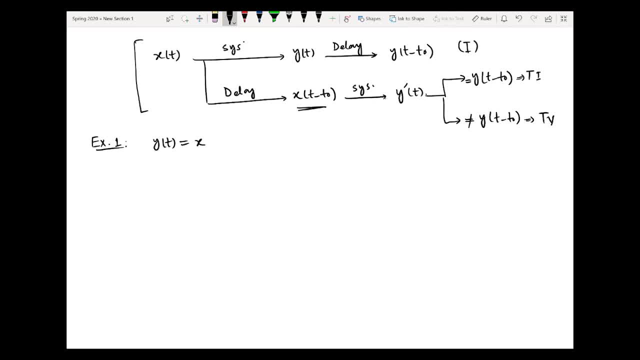 example is: let's say, y of t is equal to x of t minus 1. now, if you take the input as x of t, now I am going to verify it through this one, the block diagram shown above. so I will pass x of t through the system and after passing through the system, I am getting the output, which is y of t is. 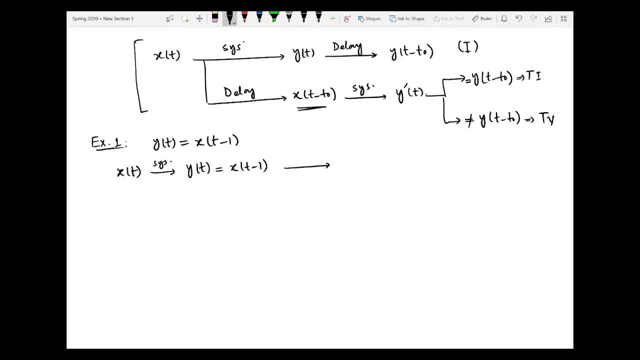 equal to x of t minus 1. and now I will pass it through a delay, delay by t naught. so when I pass it through, the delay, t naught and the output will be x of t minus t naught minus one. so I will introduce a delay equal to t naught now. now I have to check the second branch by reversing. 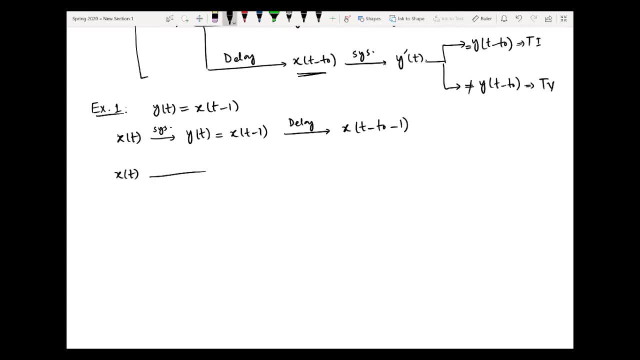 the order. so again taking the input as x of t, now passing through a delay, when i delay it, so it will become x of t minus t naught, and then I will pass through the system in the reverse order. so now, if I pass through the system again, we have to see the functionality of the system here. the functionality. 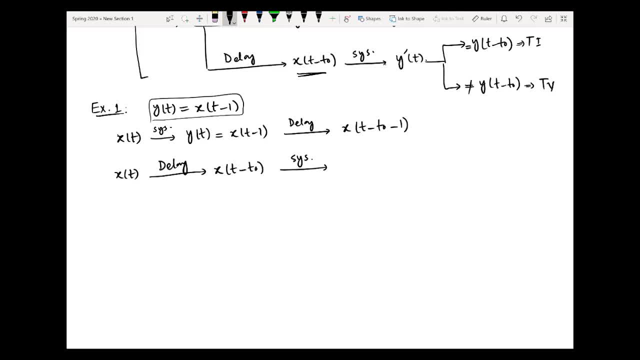 of the system is: if you look at this particular equation, the functionality is simply that this system is introducing a unit delay in the applied input. Here the applied input is this: So the system will just introduce a unit delay in the input to result the output as x of t minus t0.